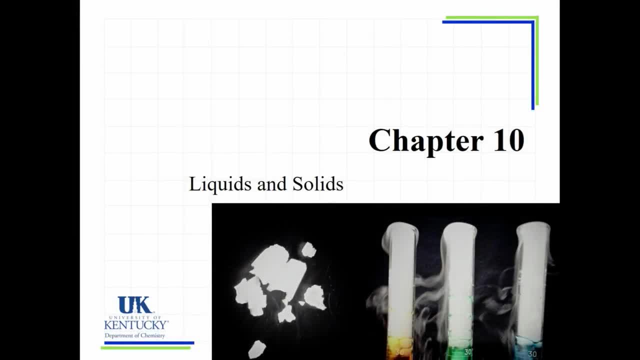 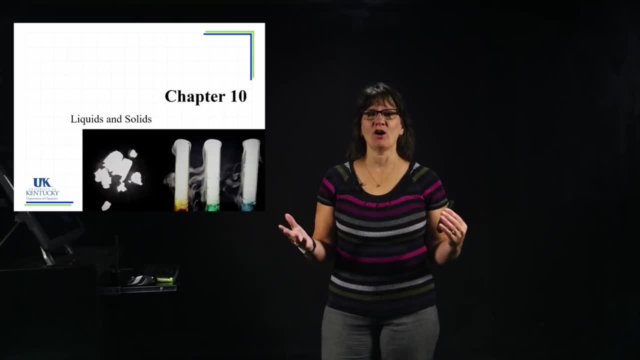 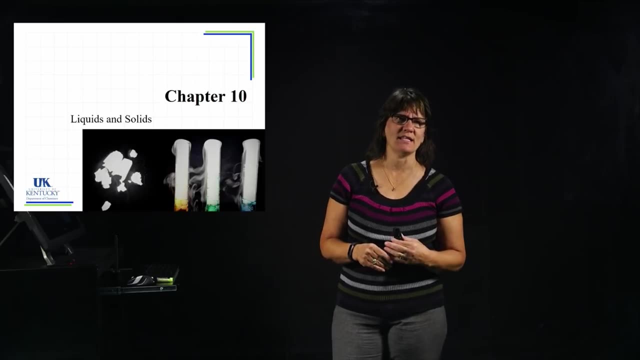 So we've just spent a whole chapter talking about the gas state and there's a whole lot of laws- Boyle's law, Charles law, ideal gas law- a lot of calculations that we can do that interrelate how gases behave. Now we're going to look at the other two states of matter. We're going to look at the 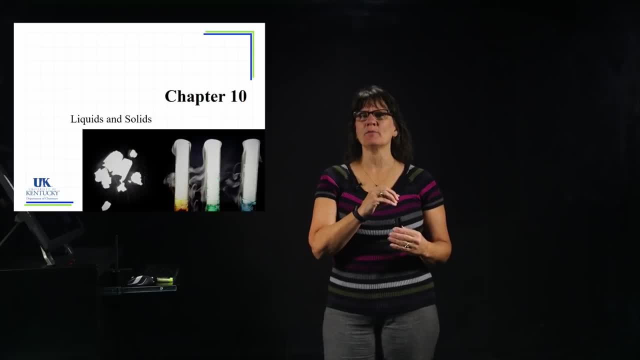 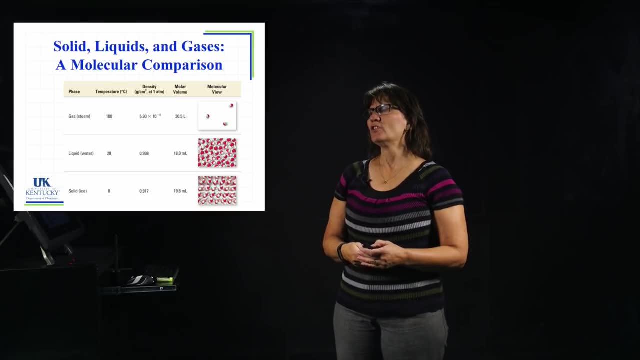 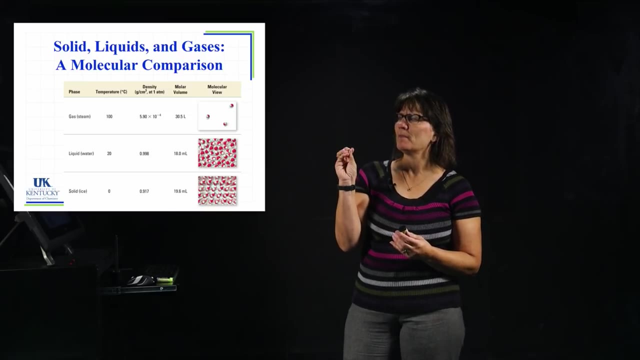 liquid state and the solid state, and we also spend time talking about the inner conversion between those states and include gases when we have those conversations. So let's just look at the three states here for just a minute as a group. okay, So we see on the screen there: the gas, the liquid. 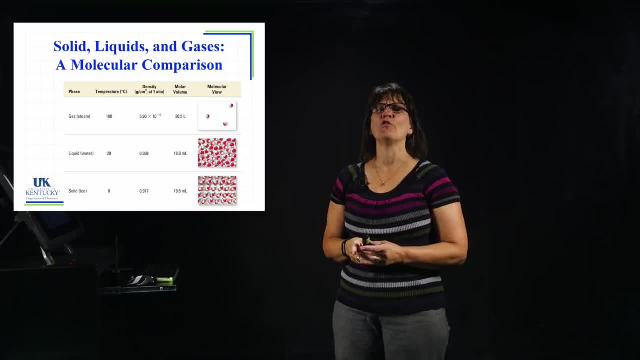 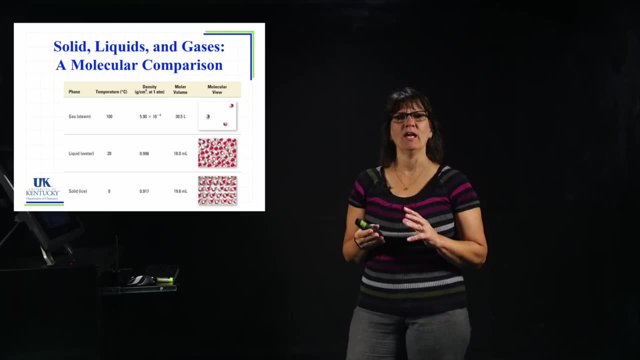 and the solid, and we have some properties given to us for water. Now I don't want you to memorize those numbers, but I do want you to kind of look at the values and we can draw some conclusions about the difference between the three states, what they're doing on the molecular level. So we 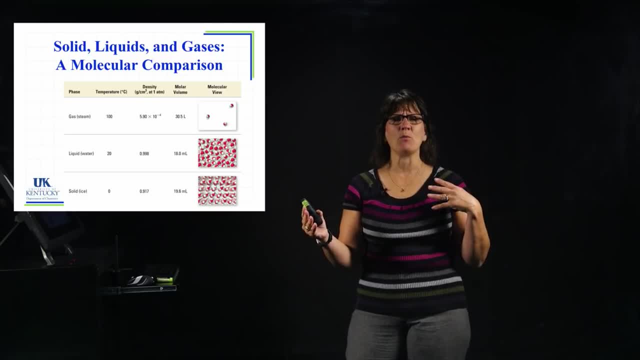 know how, what a solid is, a liquid is and a gas is. by way of you know a solid and a liquid. So solids have a defined shape and a defined volume. Liquids have a defined volume but not shape. They can take on the shape of their container and gases expand to fill whatever size or shape container. 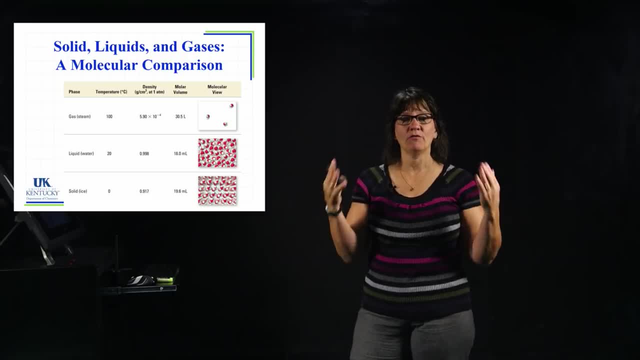 it's in. So we know that. that is how we, on the macroscopic level, on the level that we can see, we define those three states. But let's look down in the molecular level and let's start looking at what's happening with the molecules. So let me look at this a little bit and let's do some comparisons. 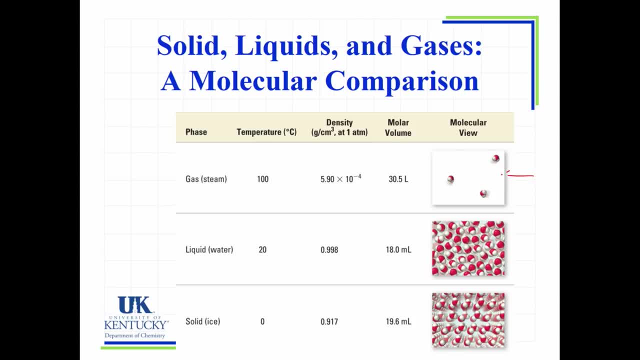 You can see on the molecular level that the gases are very, very far apart. Now this is not even to scale here, because if the molecule was that big, the next largest, the next one wouldn't fit on this screen anywhere. But there's great distances between them In the liquid state they are touching. 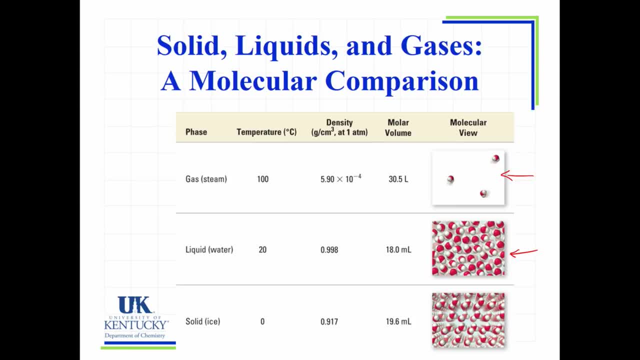 each other and they're moving about, able to move past each other and flow past each other, And in the solid state, they are packed in tightly as well, but cannot freely move past each other. The big difference between these properties is in their density- The density of liquid water and 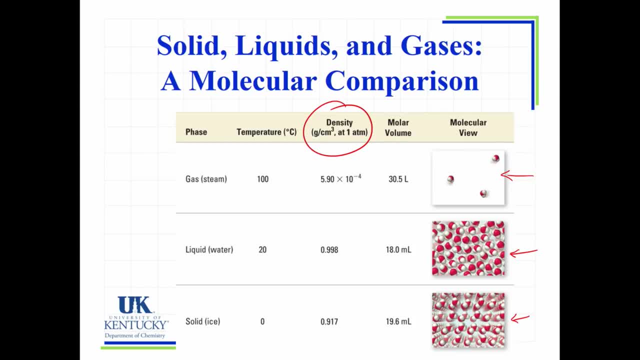 ice are about the same, but when you get down to that of a gas, it is way smaller. and this is going to be true for all gases. All gases will be way, far, far less dense in the gas phase than they are in the liquid, in the solid phase. Now, in terms of the density of liquid, 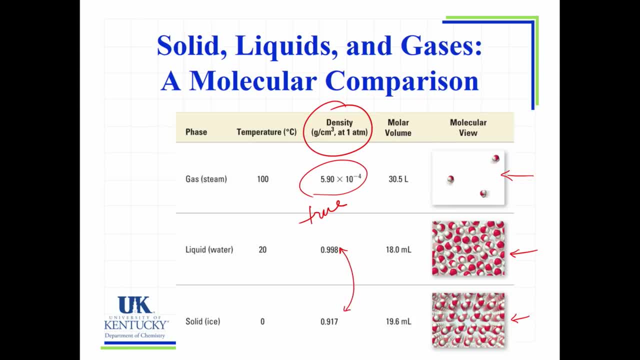 water and solid ice. okay, the fact that ice is less dense than water is very unusual. Okay, it's very unusual for that to be the case. Most solids are more dense and would sink in their liquid state, but water doesn't do that. But again, this one is the one that we need to always realize. 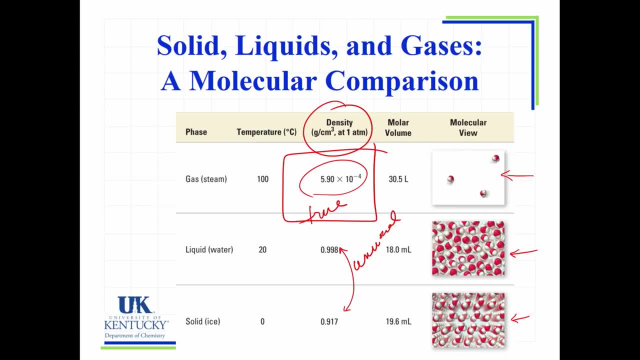 is going to be true. Now, that is just some general properties about solids, liquids and gases. I really want you to take a look at that and see if there's anything else that you want to know. I want you to think about that thing that I've got a box around and what we see on the molecular level. 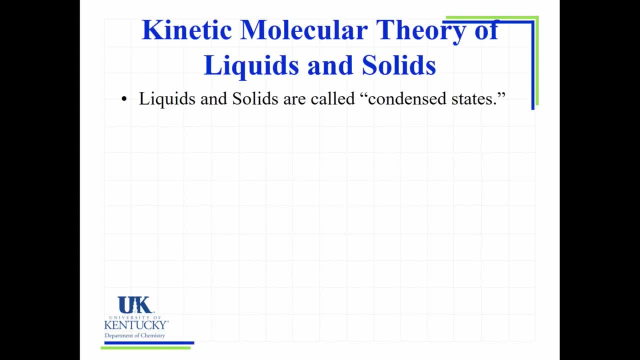 So what was going to make the difference between these things? We're going to get into the kinetic molecular theory of liquids and gases, where we talked about this, for I mean solids and liquids. We talked about this for gases already, but what we know about solids and liquids is they're considered 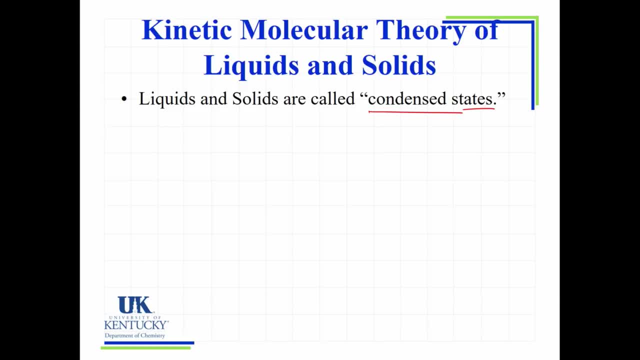 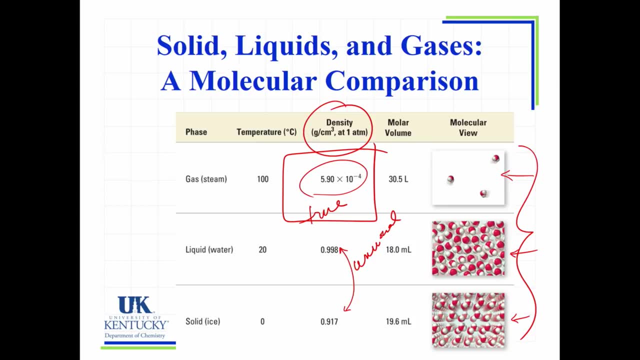 the condensed state because they are packed very, very closely together. Once again, if we go back to what we saw here, it's condensed because they're very, very close together, pushed closely together. There's an attraction that's holding them together. we're going to talk. 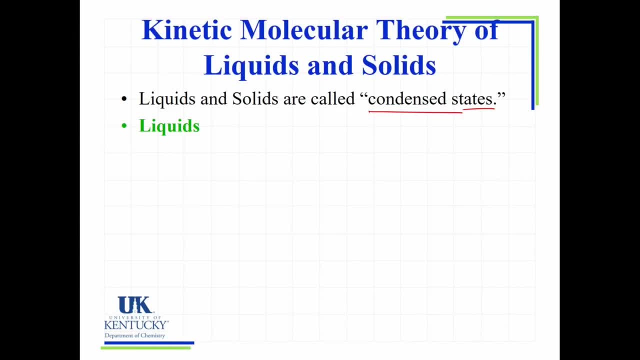 about here as we go on. Okay, so it's called condensed states, The liquid state. we see that the molecules are close together. there's very little empty space. it's difficult to compress, it's difficult to make them get into a very much smaller space than they already are. 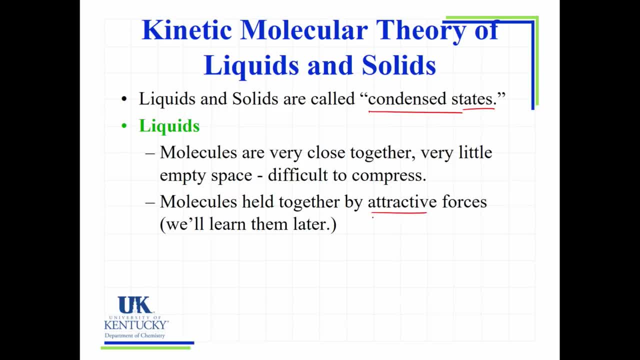 Now, what we're going to learn about today is attractive forces that hold these things together. If they're very, very close together- which it says they are, they're very close together- there's something that's holding them close together, and that's attractive forces. We already knew this from way back in chapter one. 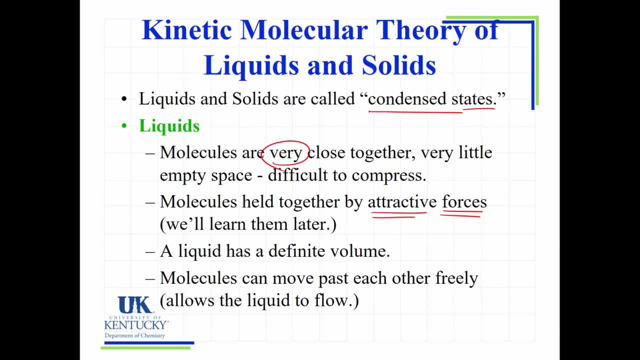 liquids have a defined volume and in terms of what they're doing in the kinetic molecular theory, let's think about those words: molecules movement. This is, the molecules are moving. Okay, so how do they move? In the liquid state, they can move past each other freely and this is what allows liquids to flow. 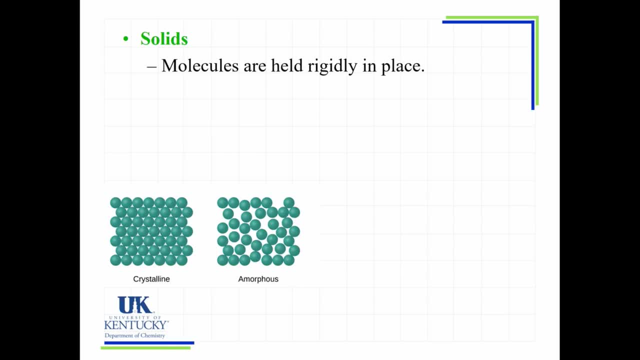 Now a little bit about solids. they're rigidly held in place. Now, they might be rigidly held in place in a very organized way or a disorganized way, but their neighbors stay their neighbors. They're even less compressible than liquids, meaning you can't push them any closer together. 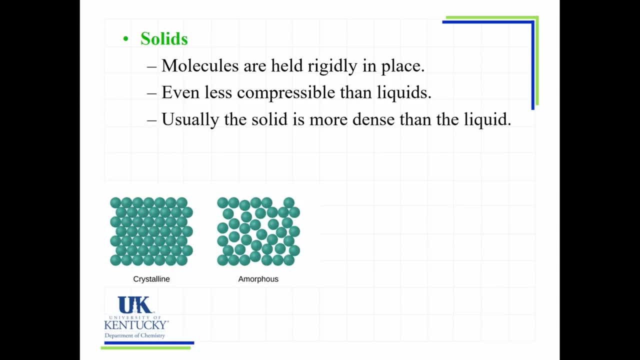 you start smashing on them. they just change shapes, if they can. Usually, like I said in the first slide, usually the solid is more dense than the liquid. They get compacted even more tightly together and this makes them more dense because they're packed. 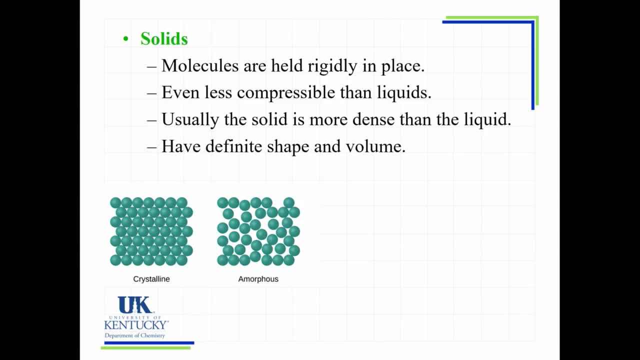 more tightly together. and again, what we learned way back in chapter one is that they have a definite shape and a definite volume. Now, what we see as an image on the screen here is the difference between what's called a crystalline solid and an amorphous solid. 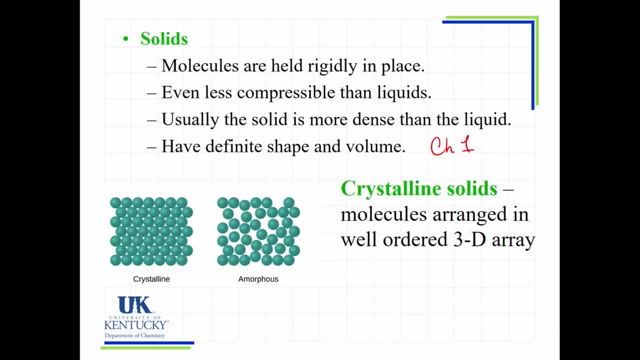 So a crystalline solid is going to have a molecular arrangement that's very well organized, very a strong order to them. So we see that happening in a two-dimensional array, but this is going to go back in three dimensions as well. So the neighbors are going to be nicely organized. 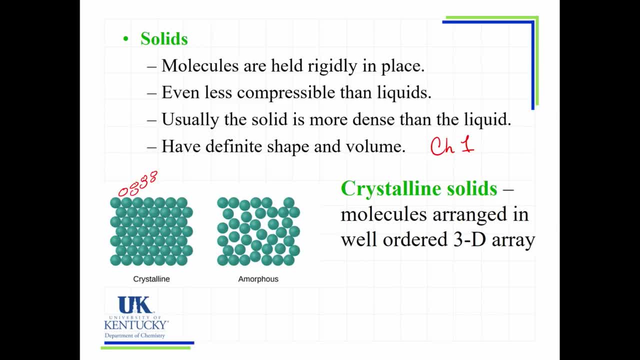 and packed together. There's a lot of different ways they are packed together, but we'll learn about that much later. So we have our crystalline solid and if there isn't this well-defined three-dimensional order, they are called amorphous solids And amorphous solids. really, that's all we're going to say. 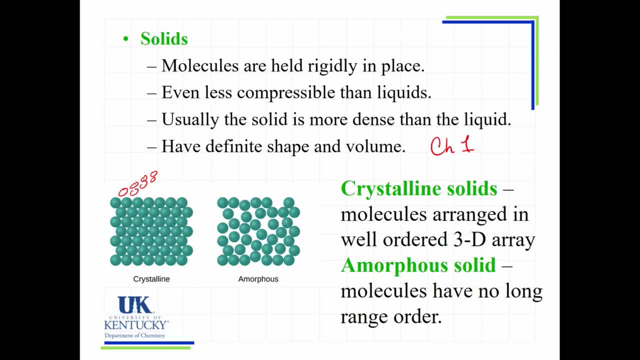 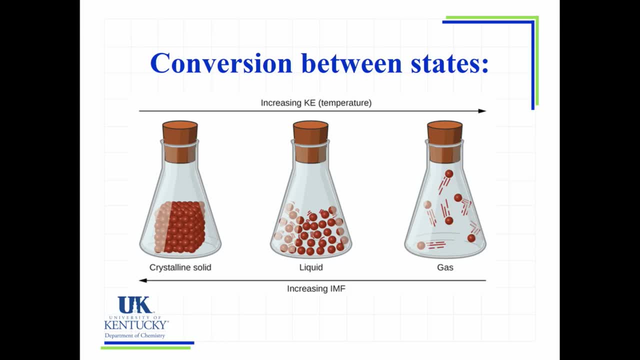 about them. They don't have any long range order. We'll talk more about the crystalline structure as we proceed through this chapter and as well as chapters in later semesters. Now I said we're going to talk about the three states of matter. we're also going to be talking 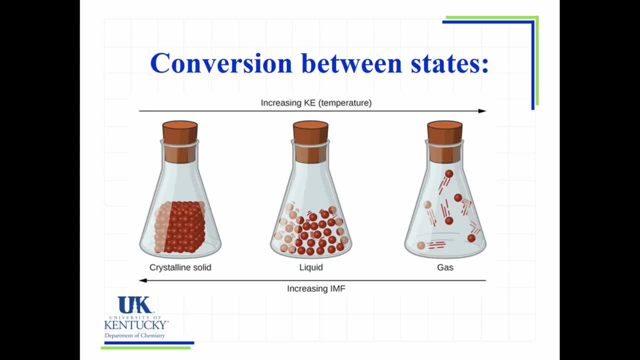 about the interconversion between those three states. So we're going to talk about the interconversion between those three states, three states of matter. so we need to keep in mind how we interconvert. if we start with a solid, let's say, for example, we start with ice, we know that. if we